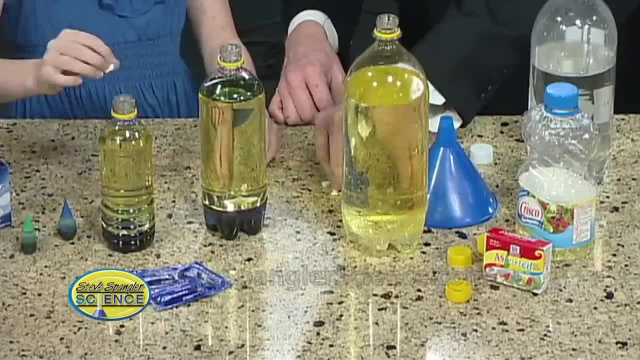 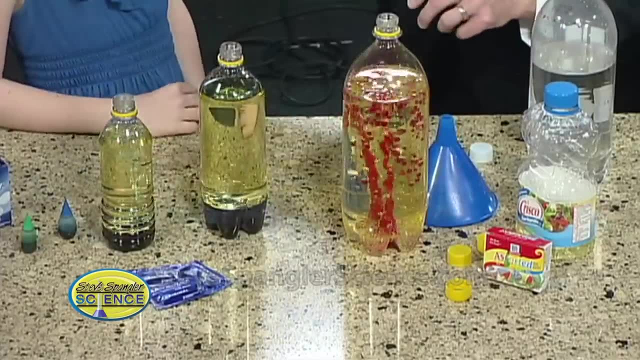 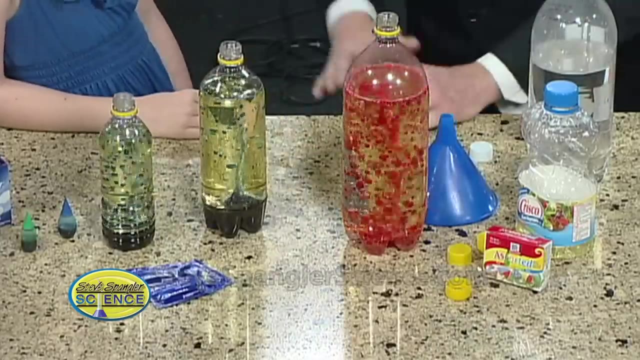 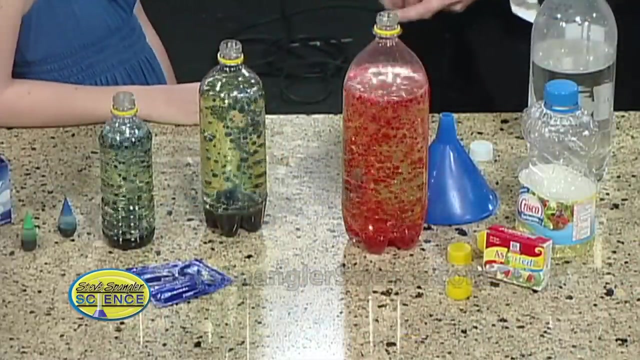 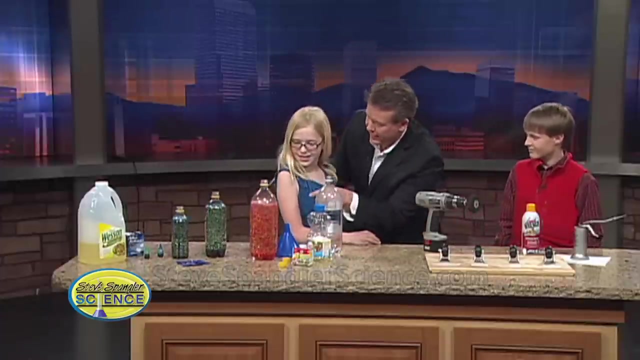 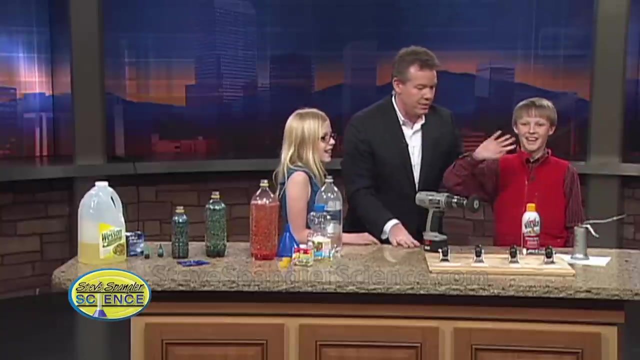 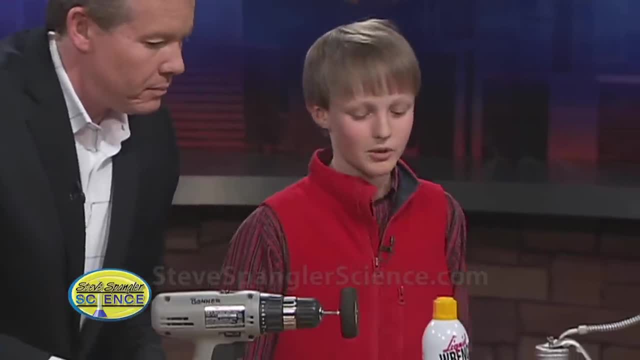 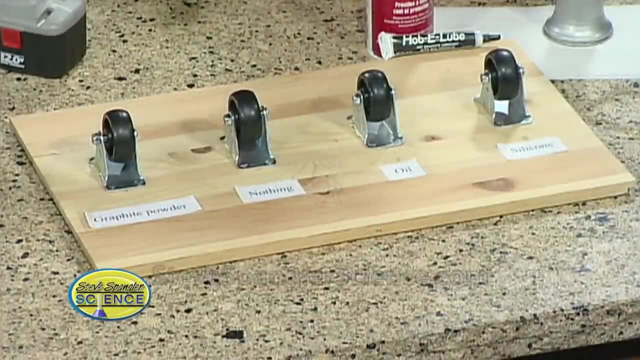 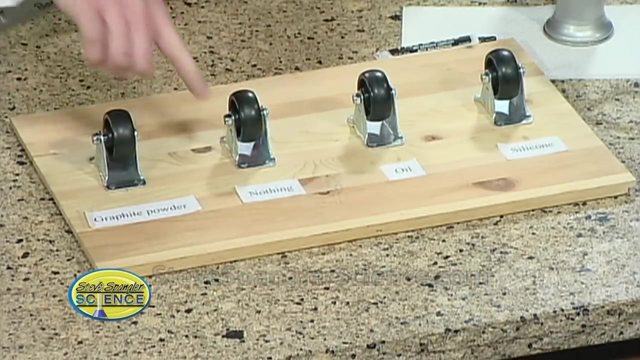 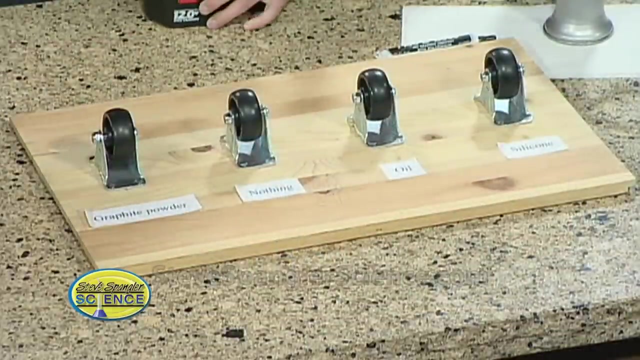 I've got the makings of a great experiment. what's going on? what are you testing? well, I want to see which lubricant would make a wheel spin the longest, and I had found out after doing mini-test that graphite powder was the winner. graphites the winner, yeah. so show me the test way, because I thought that was ingenious. show everybody what you did. you, you put graphite powder on this one, nothing oil and in silicone. then show me the test. so I went for three seconds and let it spin good, and then see how long it's weeks. but dual mall, would you do that? so all 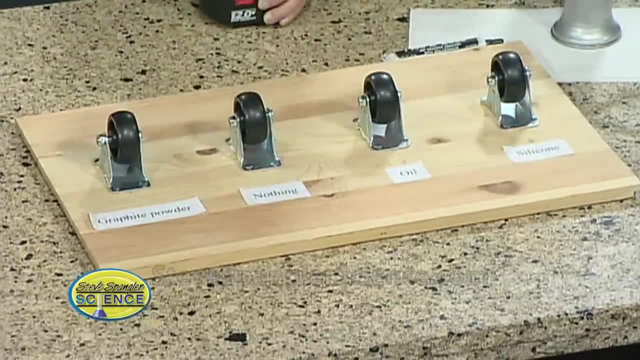 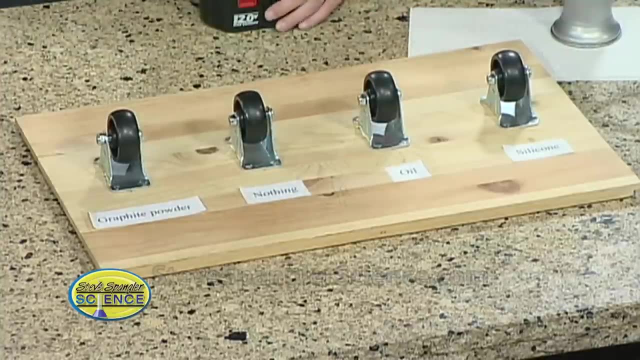 and this one was just oil, and then you had a really controlled situation because you did the same amount for each one and then tested to see and the winner is graphite powder. so this is what we need to be using. so i'm going to sneak out to mark kubrick's car and you just put a little bit. 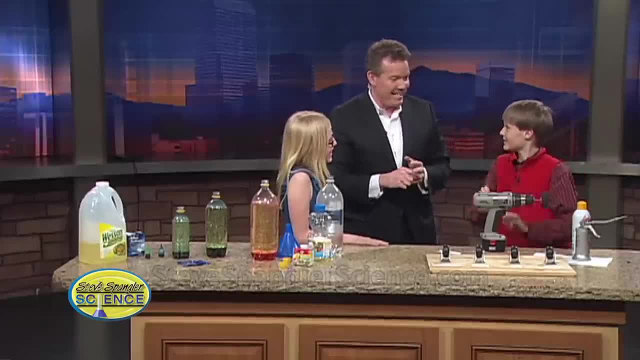 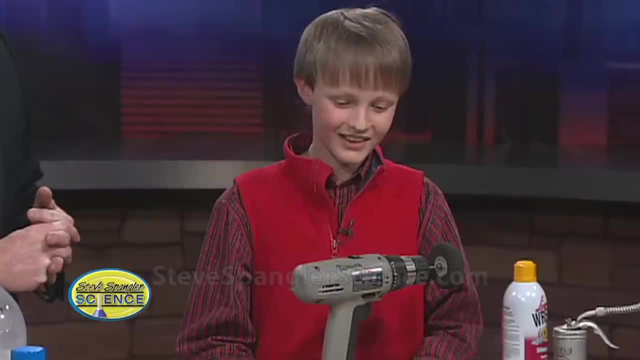 there and then it's just going to go and go and go. right, it's absolutely right. what's the one thing that you learned by doing the science fair? what was the one takeaway that you always remember doing the science fair? well, hard question: which lubricant is going to work? i would say i hope. 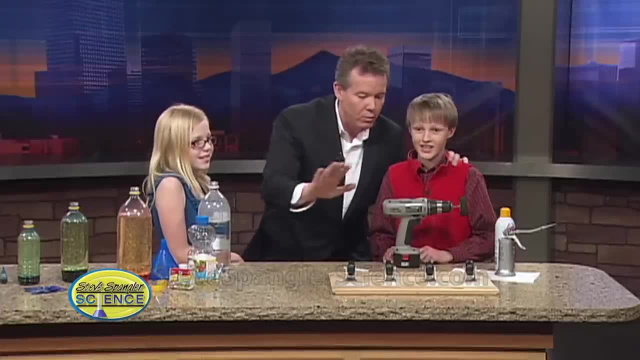 that you learned a sense of wonder. did you learn that? okay, look in the camera and say: i learned how to wonder, i learned how to discover, i learned how to discover and i had fun at night news. how's that?